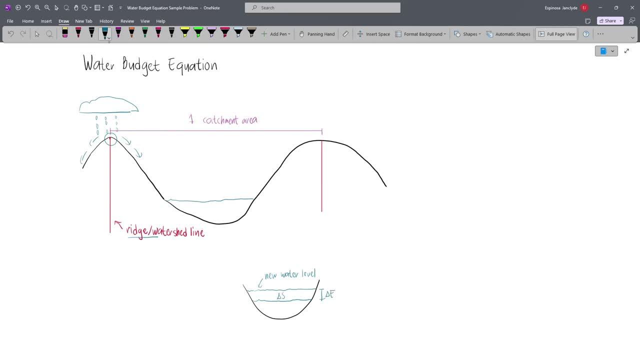 the change in elevation, If we will just consider the depth of the water. Now, again, in this area there may be an inflow or outflow of water, But in majority of the cases our inflow is mostly due to precipitation. 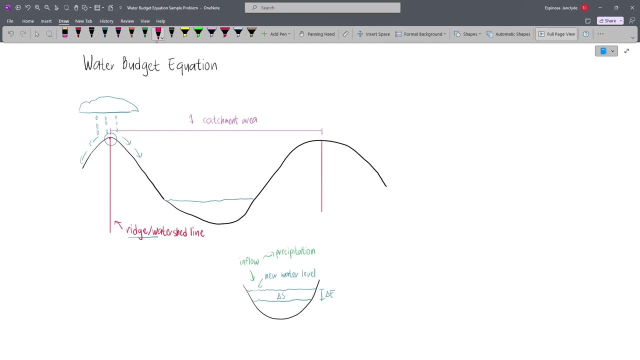 However, outflow will also occur Now in our hydrologic cycle. this outflow may be due to evaporation, transpiration, surface runoff, or sometimes this outflow may be caused by infiltration or groundwater flow, if these are flowing out of the catchment area And 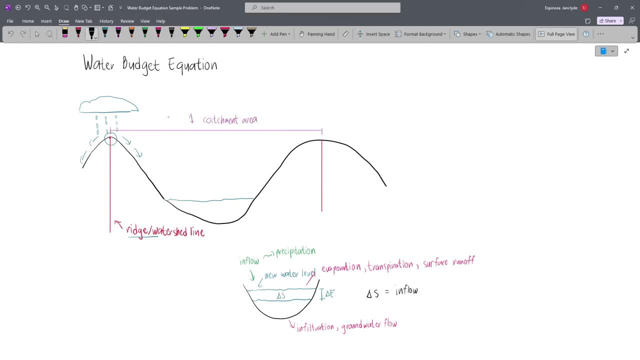 so, essentially, delta S is just equal to the inflow minus the outflow, And so, since in most cases this is just the precipitation, we can describe delta S as precipitation minus the outflow, which are runoff groundwater flow and outflow. 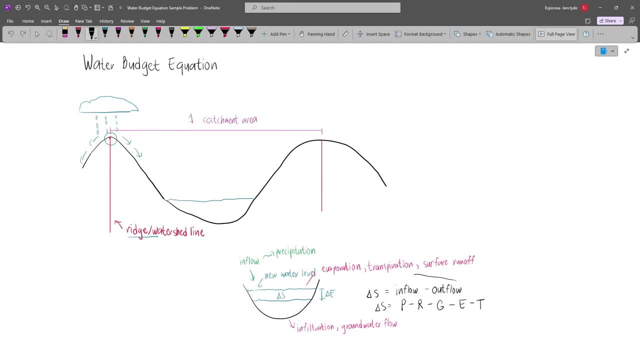 And so this is basically our general formula. So if you know this, it's your choice whether you want to memorize this one, because you can always just use this in any type of problem. Again, P stands for precipitation, R is for runoff, G is for groundwater flow, E is for 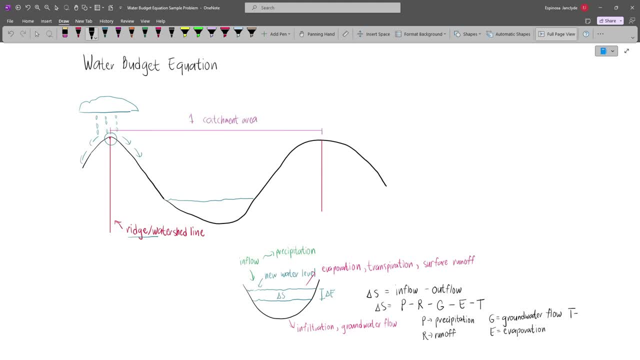 evaporation, and then T stands for transpiration. However, delta S may also be expressed in terms of elevation, still be delta E is equal to inflow minus outflow. However, this is in terms of distance, while this is in terms of volume. Next, we also have the rainfall and runoff relationship. 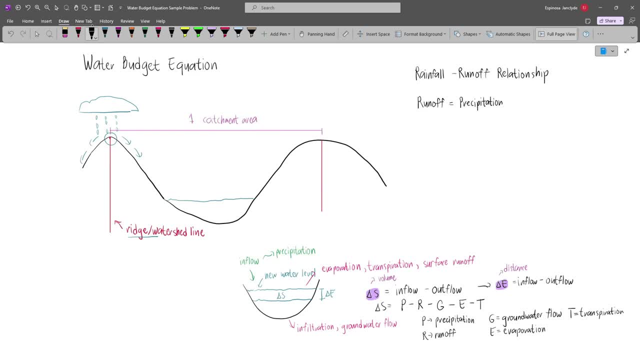 wherein runoff equals precipitation minus all the losses due to infiltration. Now these losses cause an addition to soil moisture and groundwater storage. And then another important equation is the runoff coefficient: whch is runoff divided by rainfall. Now rainfall is just due to precipitation, And so this is an important formula, and also this one: 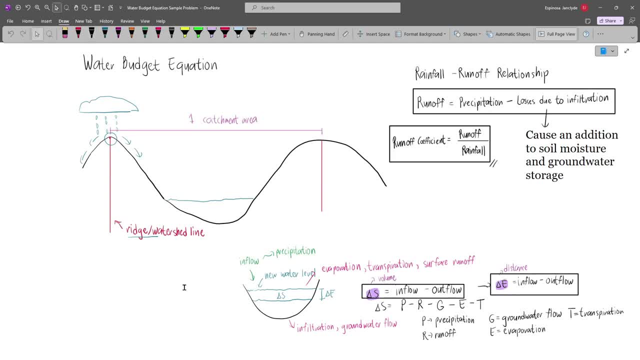 as well as these, And so, to better understand these equations, Let's try to solve some problems. However, note here that the new water level may rise or it may also fall, Depending on the situation. if inflow is larger than outflow, the water level will rise. However, 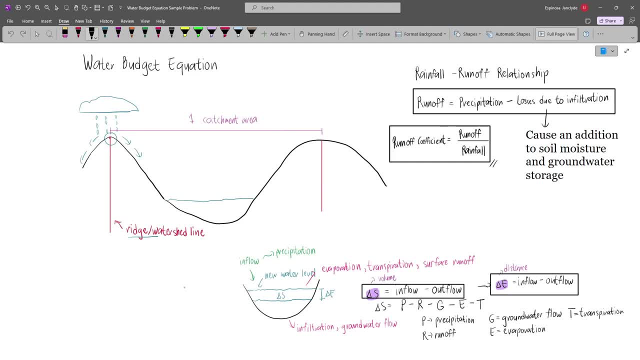 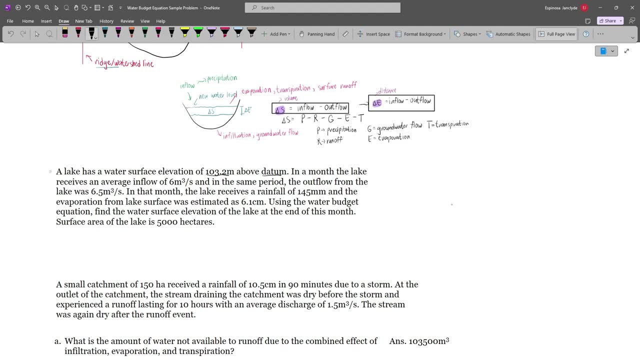 if the outflow is significantly large, then there will be a decrease the water level, and so for our first problem, we have a lake that has a water surface elevation of 103.2 above datum. now, in a month, the lake receives an average inflow of six meter cubed. 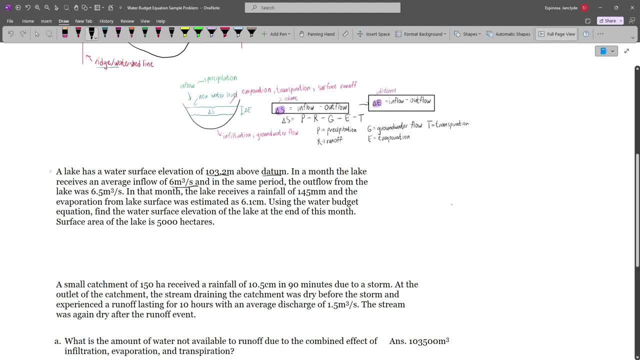 per second and then in the same period, the outflow from the lake was 6.5 meter cubed per second. now again, this is just similar to discharge, which is volume per second. now in that month the lake receives a rainfall of 145 mm and the evaporation from the lake surface was estimated as 6.1. 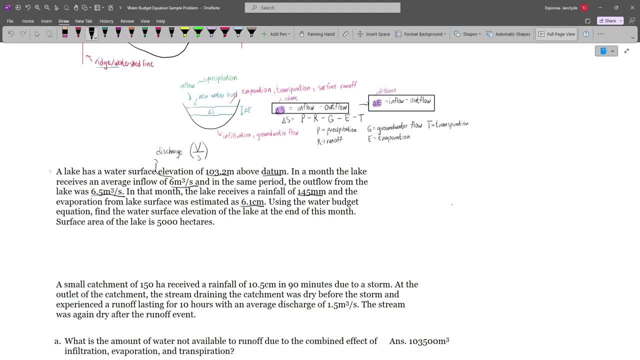 centimeters. using the water budget equation, we have to find the water surface elevation of the lake at the end of this month, and then the surface area of the lake is 5000 hectares. now it's important to note here that in our question we are considering at the end of this month, and so that 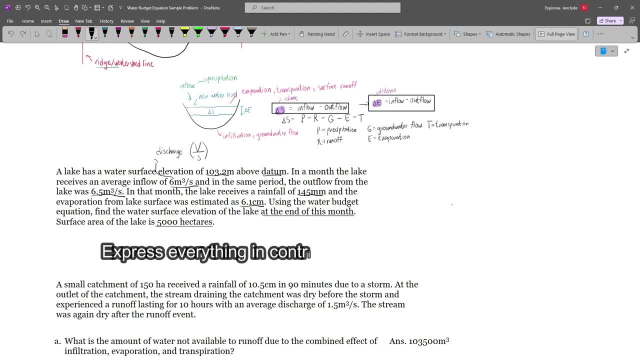 means that we have to express all of our values in terms of its influence per month. and then we also have to note that we are given the elevation, and so that means that we should use this formula, which is in terms of distance, and so that means that we should use this formula, which is in terms of distance, and so 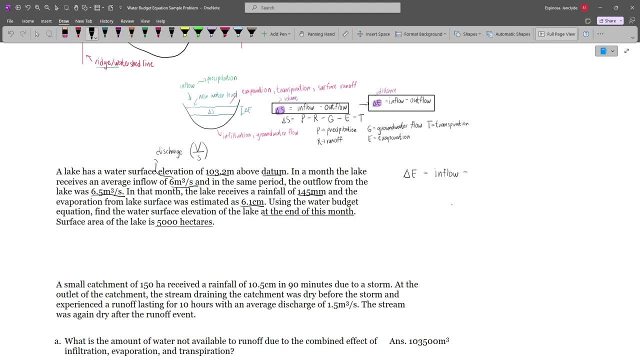 we have delta e is equal to inflow minus outflow. now our delta e is just the change in elevation, and so that will be the final elevation, which is ef minus the initial elevation. now our initial elevation is 103.2, so this is 103.2 meters, and then this is equal to inflow minus outflow. now let's 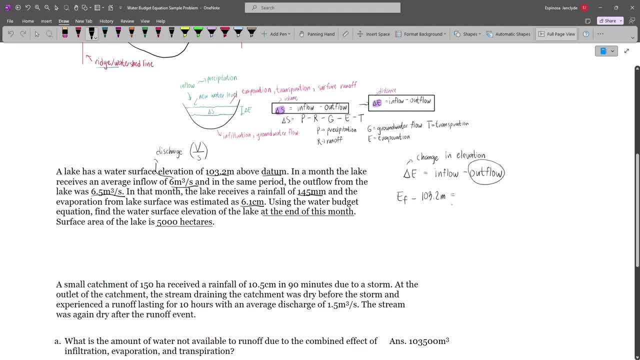 first identify what causes inflow and what causes outflow. now, in a month, the lake receives an average of 145 mm, and so this is inflow. let's color them yellow. and then the outflow from the lake was 6.5 meter cubed per second. now for outflow. let's color them pink. now, in that month, the lake receives a. 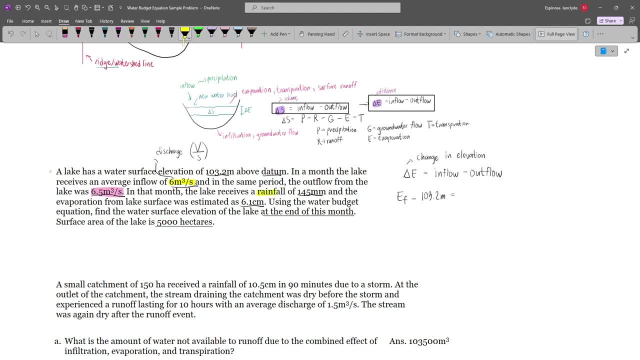 rainfall of 145 mm, and so, since this is from precipitation, this is essentially part of inflow. and then the evaporation from lake surface was estimated as 6.1 centimeters, and so we know that evaporation is part of outflow. so let's color this pink now. the surface area of the lake is 6.1. 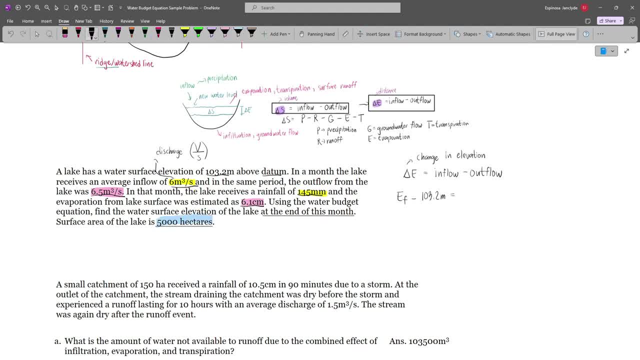 hectares. now our conversion factor for that, since we have to express everything in meters we have one hectare or ha is equal to 10, to the fourth meter squared. this is our conversion, and so first let's write our inflow. we have an inflow of 6 meter cubed per second, so this is 6 m cubed per. 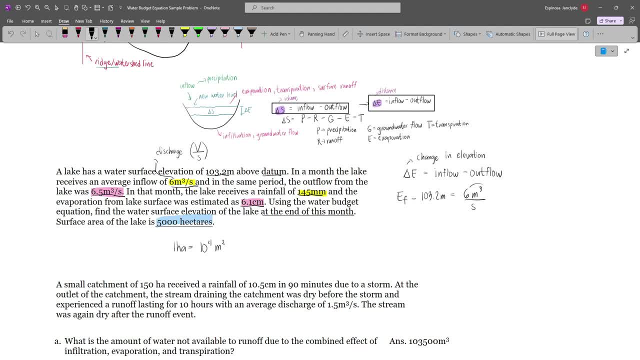 second, however, notice that this is m cubed, but we want to express everything in terms of distance, and so we will divide this by the area and so, dividing that by the area, we will get the area of the area, which is 5000 hectares. we have 5000 hectares, and then we need to convert this. 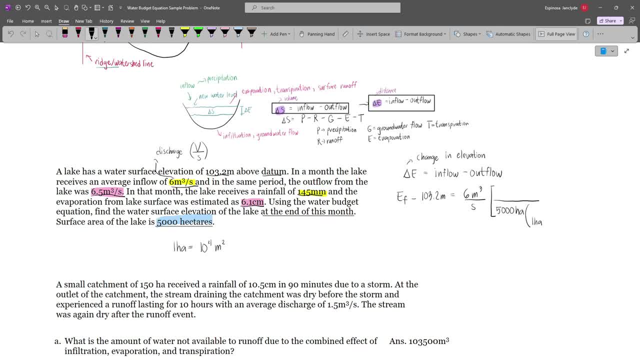 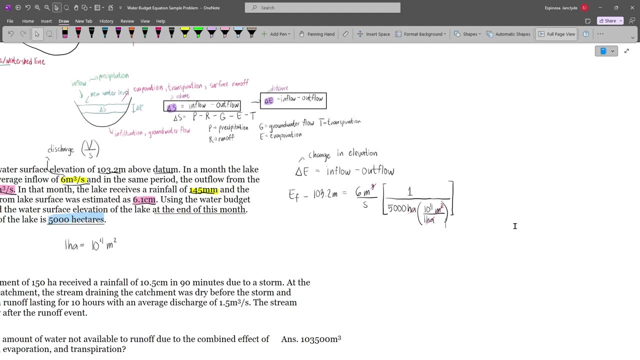 because this is m cubed. now, one hectare is equal to 10, to the fourth meter squared, and so ha will cancel, and then m cubed here will just become meter, because this will also cancel, and so we are left with meter per second. however, since we also want to express everything per month, 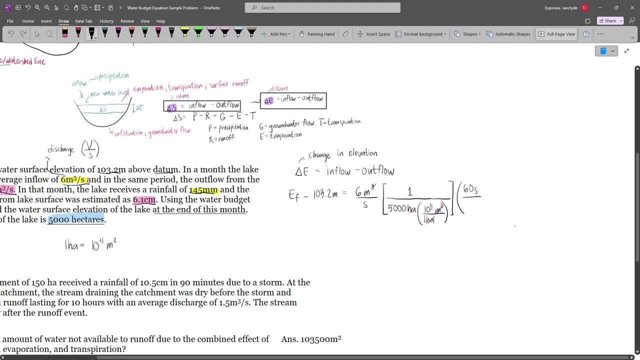 we also need to convert this now in 60 seconds. we have one minute, and then in 60 minutes we have one hour, and then in 24 hours we have one day, and then in 30 days we have one month, and so all of these will cancel, and then we are left with month. 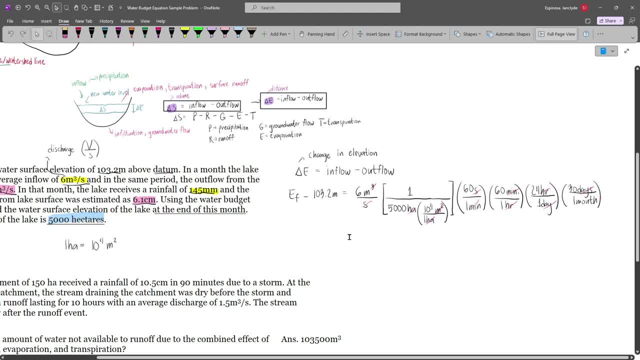 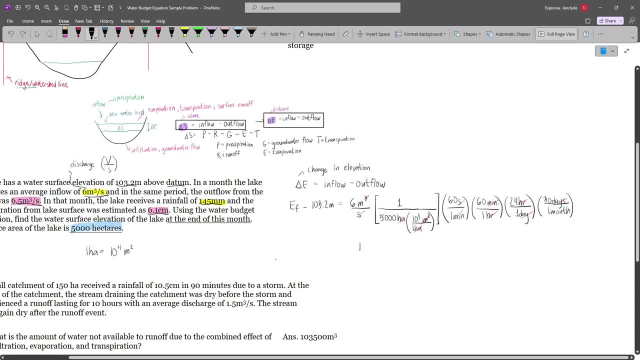 and so the unit of this is essentially meter per month, and so this is fully converted. now this is still our inflow. what is another inflow? it's the rainfall, and so that'll be plus 145 mm. and then this is per month, because it says here: in that month the lake receives this. 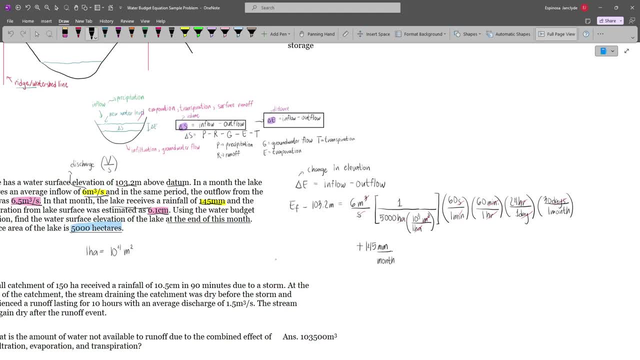 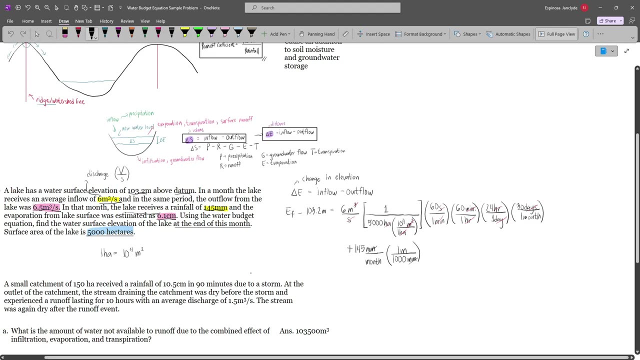 value of rainfall, and so, since this is already per month, we only need to convert mm into meters. now, 1000 mm is equal to one meter, and so these will cancel, and then we are left with meter per month, and so this is now okay, and then next we have to subtract all of the outflow. now, this is 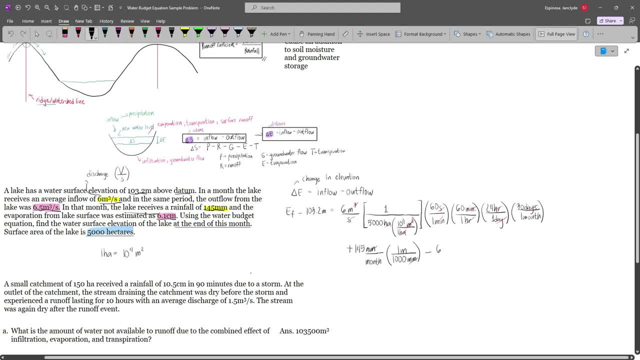 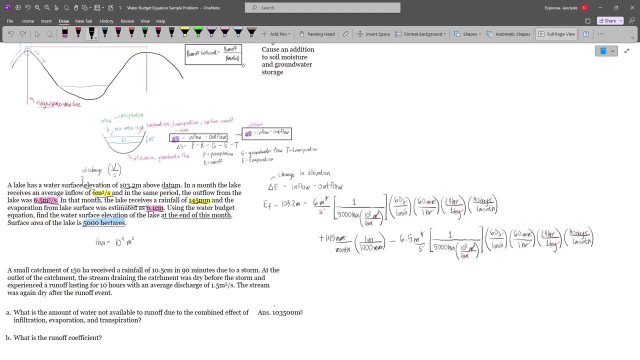 outflow. so we have to subtract that, so that's 6.5 meter cubed per second, and then let's just actually use the same conversion because we need this to be in meters per month. so let's copy this one and then these will cancel, and then next we also have evaporation, and so that will. 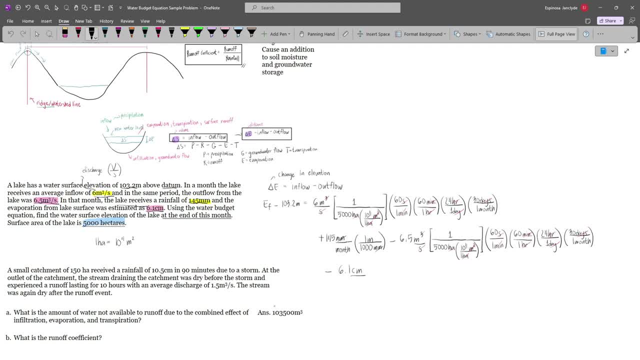 still be outflow, so that's 6.1 cm per month, and then we'll just convert this into meters, so that'll be: 100 centimeters is equivalent to one meter, and so these will cancel, and so, since all of our units are in meter per month, then we can now solve ef or the final elevation, and so we have x minus 103.2. 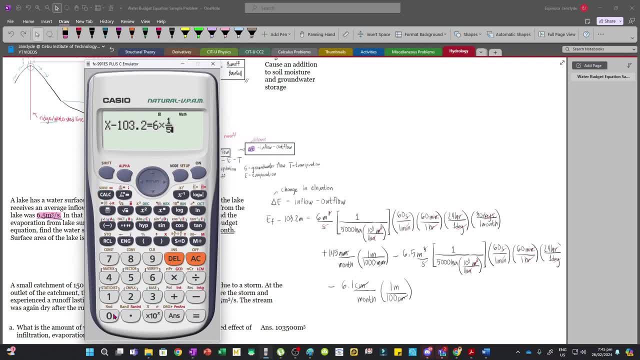 is equal to six times one, over 5000 times 10, to the fourth, multiplied by 60 times 60 times 24 times 30.. now, since our conversion factor is the same for this one and this one, we'll just actually factor them. so this will be 6 minus 6.5. now, this already accounts for this one and this one, and so we will. 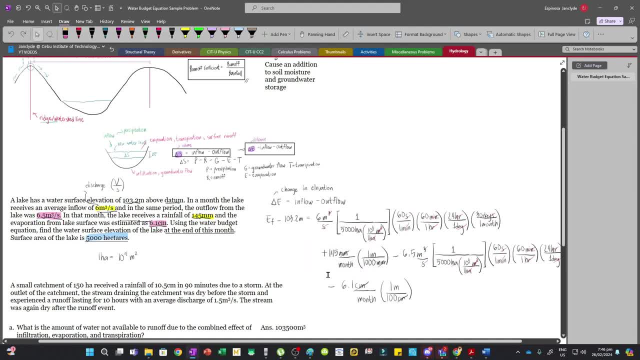 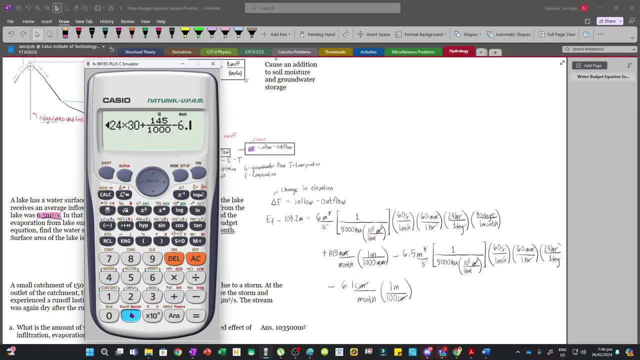 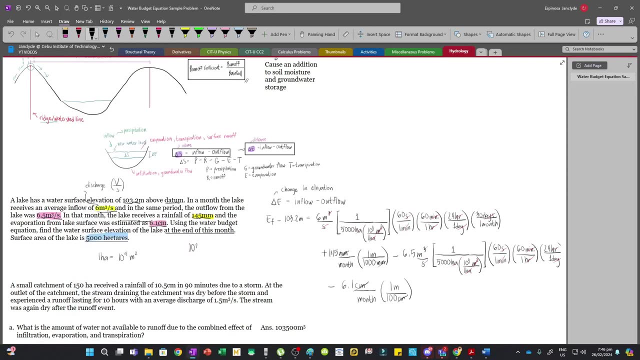 just actually consider the remaining ones, which are this one and this one. so we have plus 145 divided by 1000, and then we have minus 6.1 divided by 100, and so, solving ef, we have 103.258. so this is 103.258. 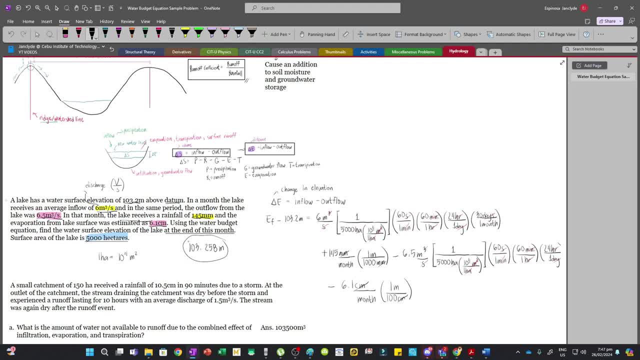 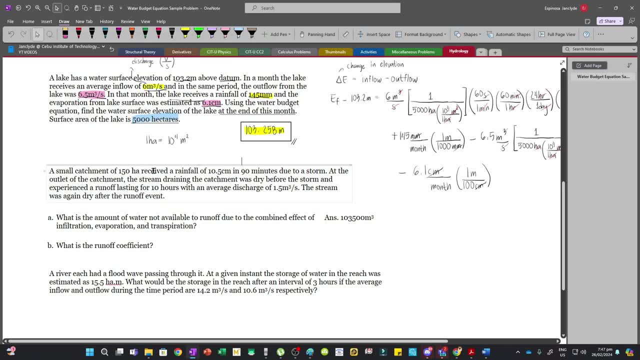 and then this is meters. now, this is the change by the end of the month, and so this is our answer. now for the next problem. we have a small catchment of 150 hectares, which received a rainfall of 10.5 centimeters in 90 minutes, and then, at the outlet of the catchment, the stream draining the catchment. 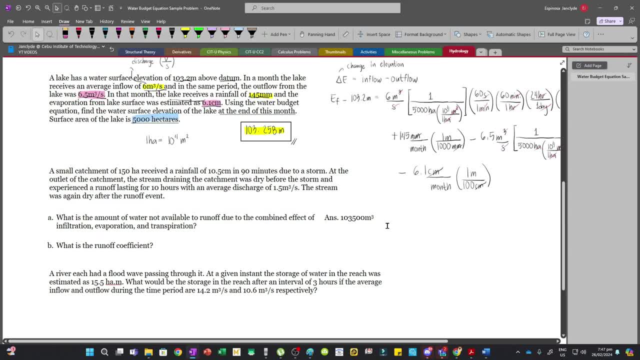 before the storm and experienced a runoff lasting for 10 hours, with an average discharge of 1.5 meter cubed per second. the stream was dry again after the runoff event. now first, what is the amount of water not available to runoff due to the combined effect of infiltration, evaporation and transpiration? 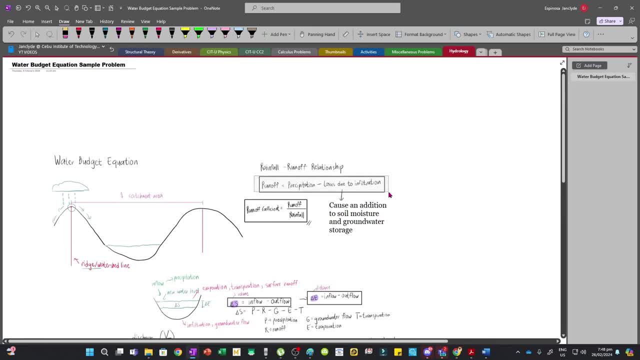 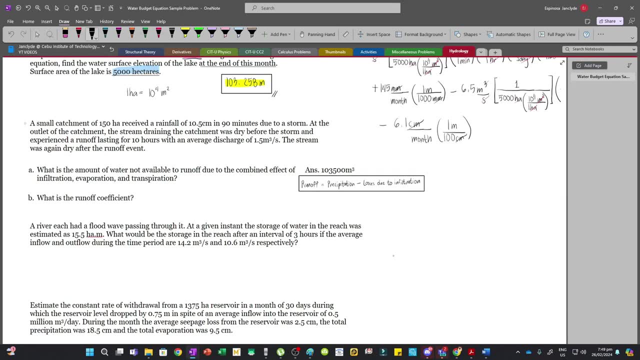 now, in order to solve this, we'll be using this equation, which is: runoff is equal to precipitation, minus the losses due to infiltration. so let's copy this one now: what is our runoff? it's actually the one. it lasted for 10 hours and this is our discharge. and then what is our precipitation? 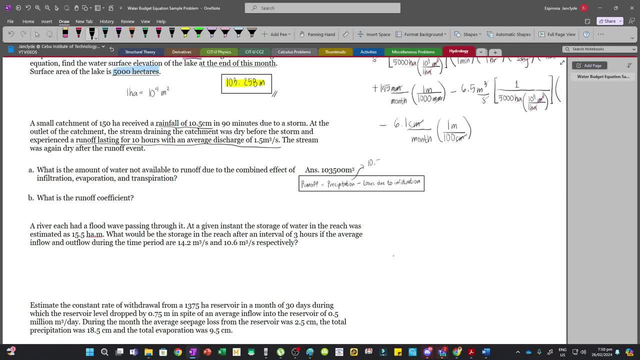 it's actually this one, and so this will be 10.5 cm in 90 minutes. however, we won't need this information, because we already have the change in elevation due to rainfall, and then we also have the area, and then runoff is 1.5 meter cubed per second, lasting for 10 hours. by the way, the 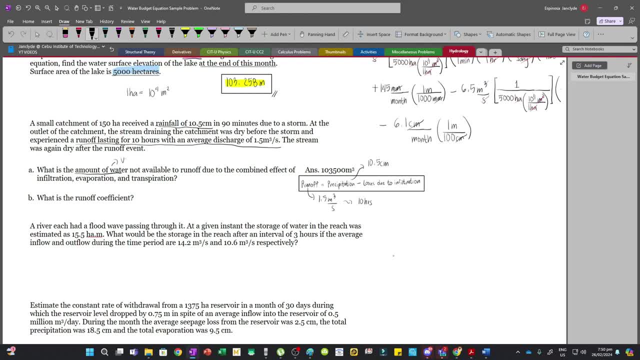 amount of water asks for the volume. so we need the volume now, first for the runoff. we would have to just actually multiply this by the time so that seconds will cancel, and then we are left with a unit of volume. so 1.5 m cubed per second multiplied by 10 hours, we can get the total. 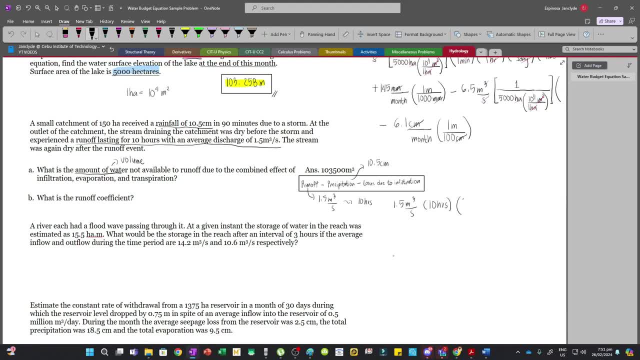 volume. however, we need to convert this into hours, and so 60 seconds is one minute, and then 60 minutes is one hour, and so these will cancel, and then we are left with meter cubed because hours will also cancel. now, this is our runoff, and so, since r is equal to p minus l, we can 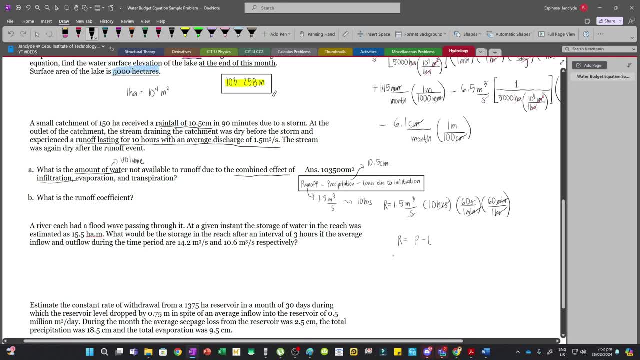 get l, which is the combined effect of infiltration, evaporation and transpiration, and so this will be 1.5 m cubed multiplied by 10 times 60 times 60 is equal to 10.5 cm, which will convert to meters, so that will be. 100 cm is 1 meter, and then we need to multiply this by the area, and so that will be. 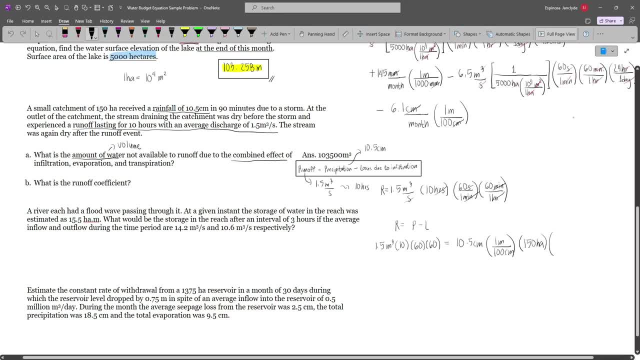 150 hectares, so 150 ha, and then 1 hectare is equal to 10, to the fourth meter squared, and so these will cancel, and also this one, and then we are left with m times m squared, which is m cubed, which is what we are looking for, and then minus l, and so, solving l, we have 1.5 times 10 times. 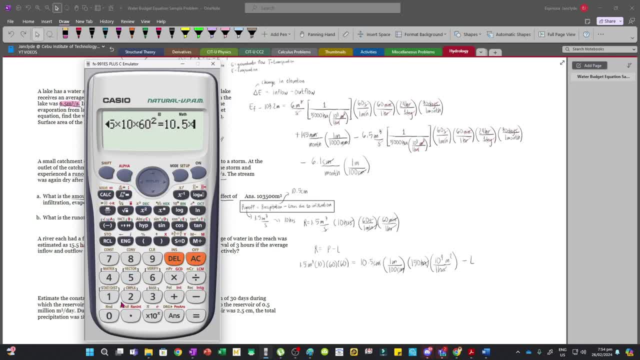 60 squared is equal to 10.5 times 1, over 100 times 150 times 10 to the fourth, and then minus l, so l will be one hundred three thousand five hundred, and so this is one, oh three, five hundred m cubed. 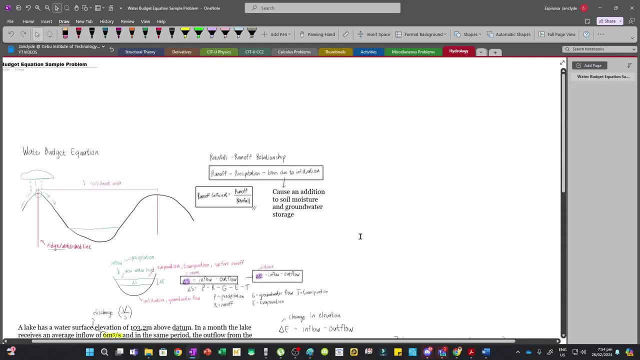 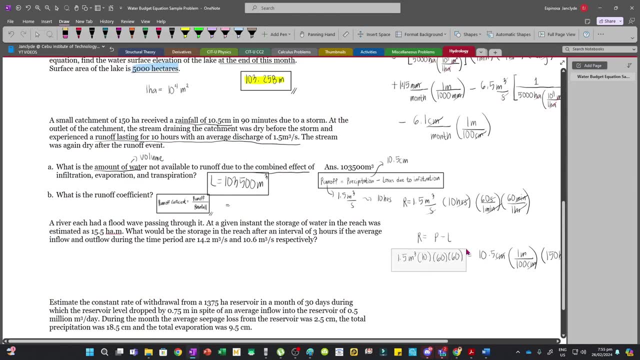 and then minus l will be one hundred three thousand four hundred, and so this is the first term for runoff and then next, if you are to compute the runoff coefficient, we need this formula: runoff coefficient is runoff over rainfall, and so this will be our runoff is this value, which is: 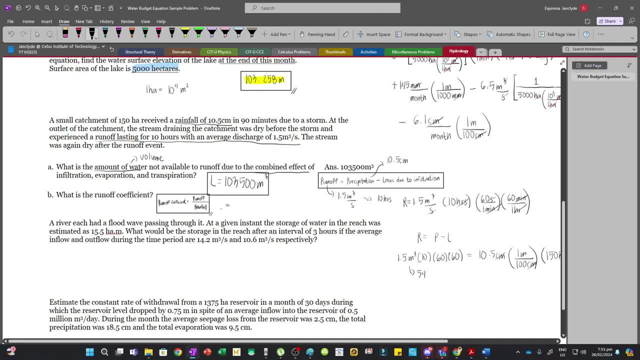 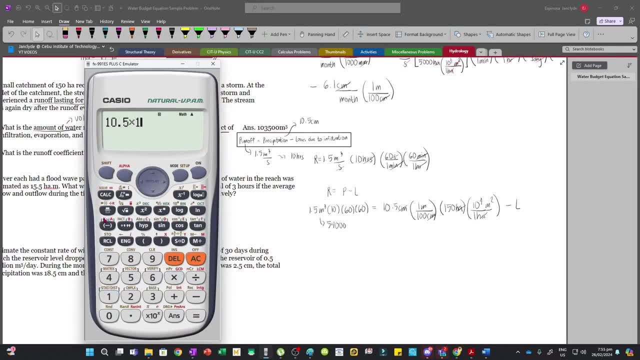 1.5 times 10 times 60, squared, that will give us 54 000, so runoff is 54 000, and then divided by the rainfall, which is this expression, now, that'll be 10.5 times 1, over 100 times 150 times 10 to the.